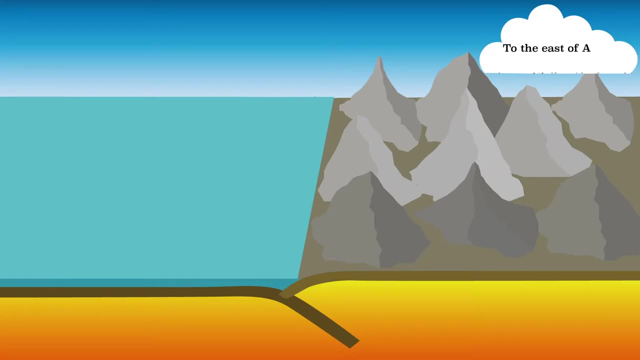 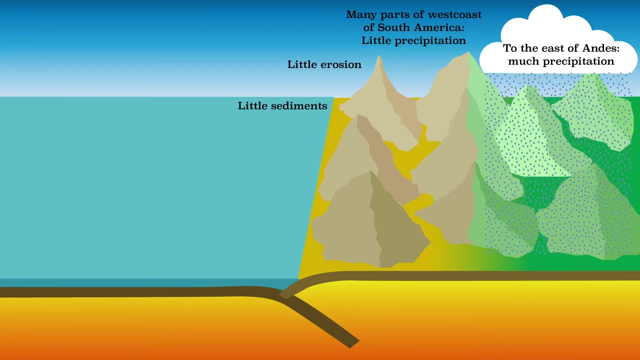 Furthermore, a large part of the west coast of South America has to deal with a dry climate, Because there is little rainfall, there is little erosion and therefore there are few sediments deposited in the deep sea trench. Sediments work as a kind of lubricant between plates. 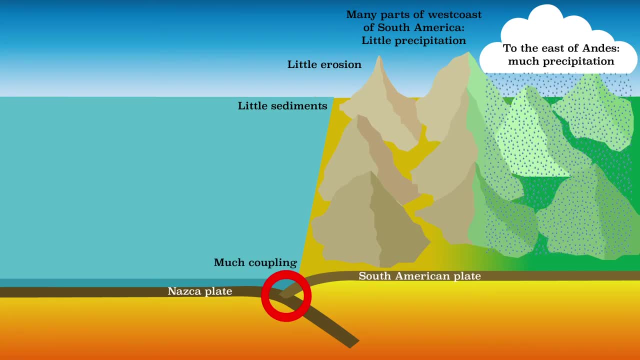 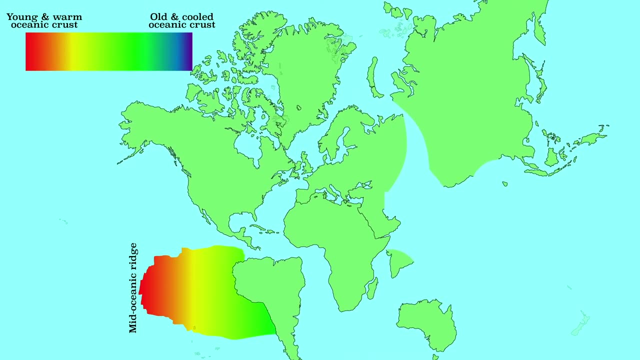 and the absence of sediments therefore ensures that there is a lot of coupling between the Nazca plate and the South American plate. A final reason has to do with the method of sediments Subduction. You have already learned that subduction occurs when old oceanic plates have cooled down. 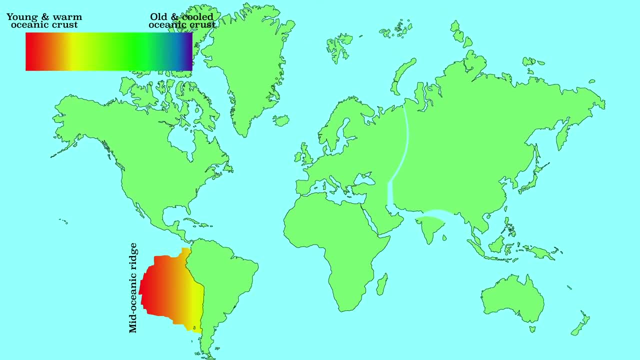 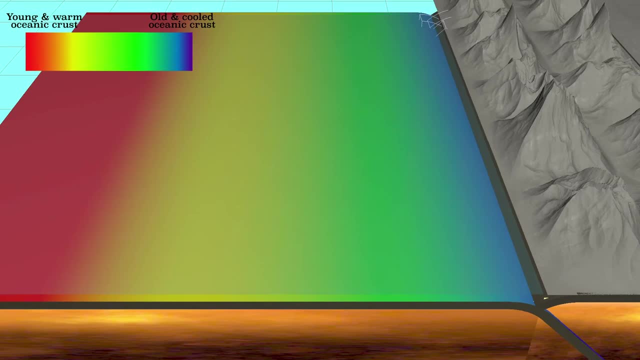 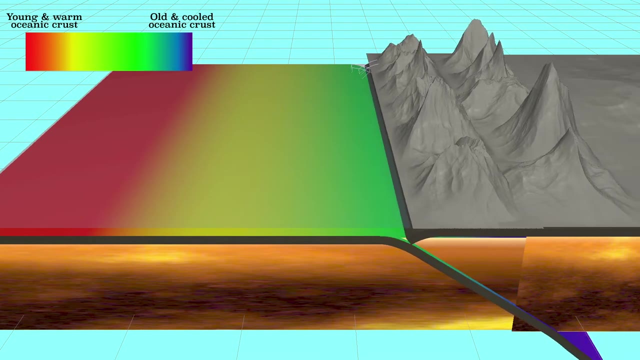 which increases the density. As South America moved westward from Africa, it came closer to the mid-oceanic ridge, where the Nazca plate originated. So the underlying plate became younger and younger at the time of subduction. At some point the underdiving plate is so young that the plate has not yet cooled down. 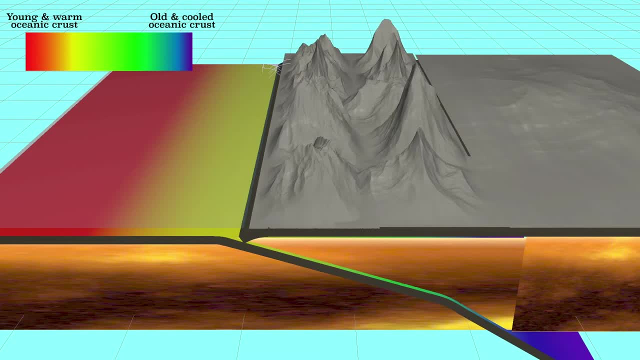 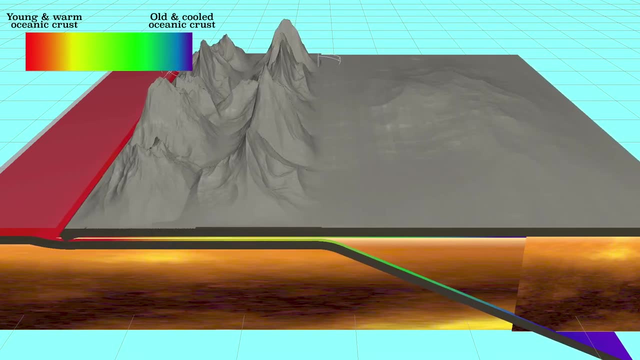 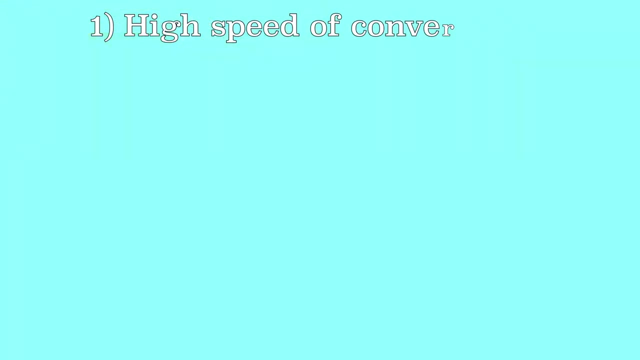 and therefore the plate has a lower density than the underlying asthenosphere. As a result, the Nazca plate does not sink down. It does not sink into the asthenosphere but remains floating under the South American plate Because the underdiving plate does not dive into the asthenosphere. this is called flat subduction. 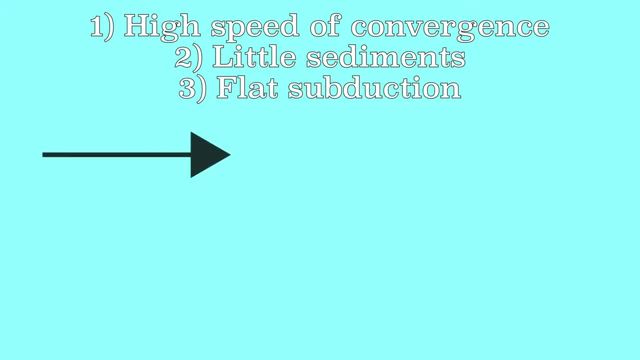 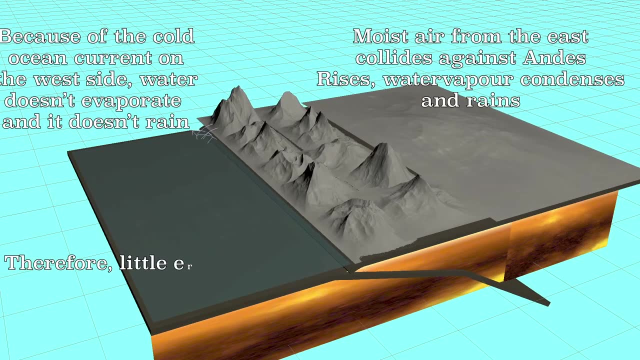 Due to the high speed of convergence, few sediments between the plates and flat subduction. there is therefore a lot of coupling. Because of this, there are heavy earthquakes and the top plate is very compressed, so that the Andes mountains could arise. 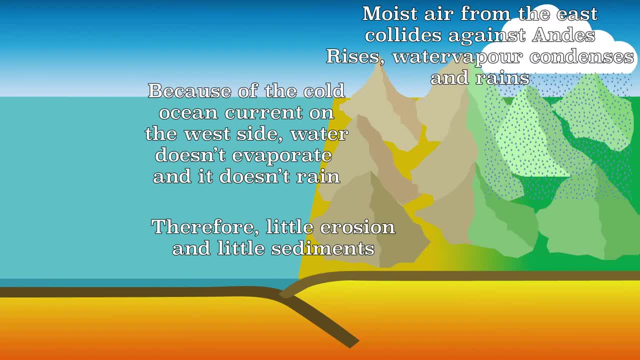 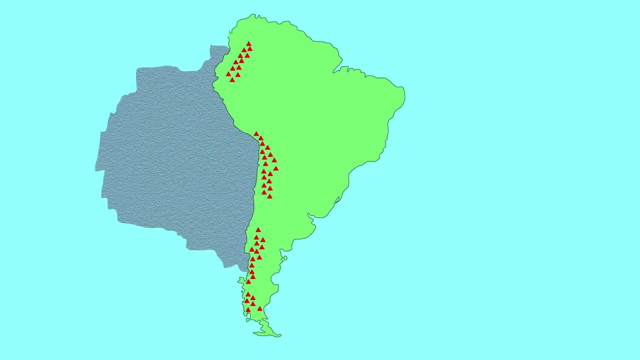 This reinforces itself Because the Andes became higher and higher from the east is blocked and therefore it rains less, So there is even less erosion and therefore less sediments act as lubricants between the plates. As mentioned earlier, there are volcanic gaps, areas where there is no volcanism. 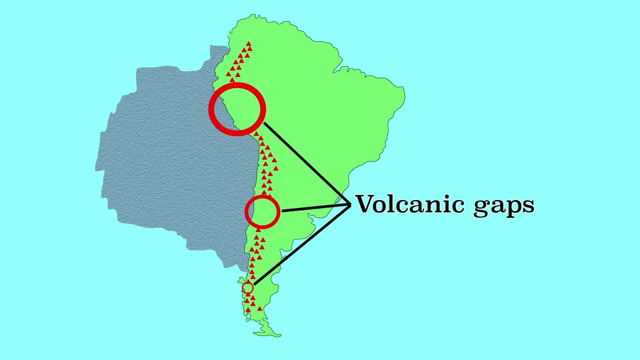 They arise in areas where the underlying Nazca plate is hot. The Nazca plate is hot, for example, because a few other mid-oceanic ridges arise crossways on the mid-oceanic ridge, such as the Patagonian gap and the Peruvian gap. 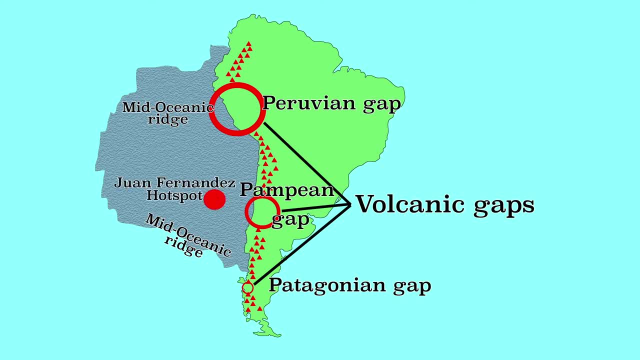 The Pampian gap was created because the Juan Fernandez hotspot heated the plate there. For these reasons the Nazca plate is hot in some locations during subduction and does not dive into the mantle, but there is flat subduction.